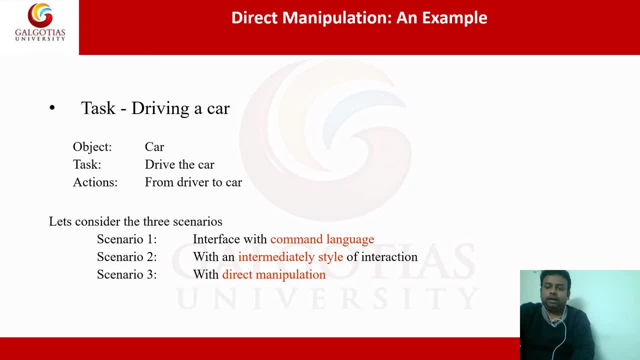 to the car. Okay, So this is a simple task. Okay, For completion of this task, we have considered three different scenarios. The first scenario is we have an interface that is a common language interface, And second is one intermediary style of interaction. 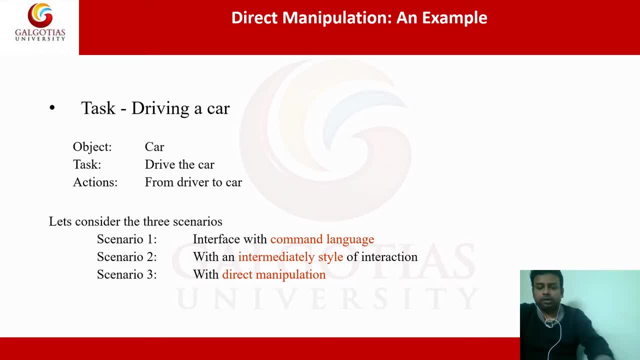 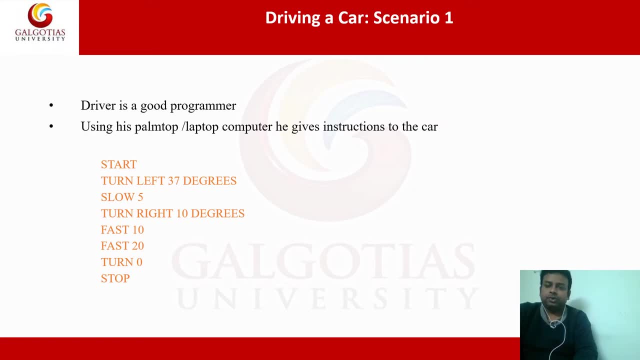 interactive interface and third is direct manipulation. So we are going for the first scenario. Let's consider: a driver is a good programmer and he is using some laptop, laptop computer, and he give some instruction to the car through the programming language And as per his instruction car is run. So he give instruction like start the car will. 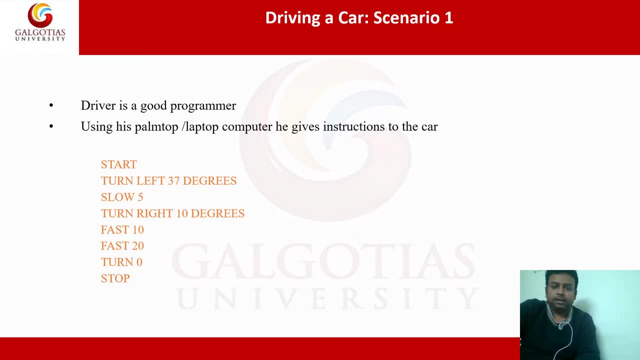 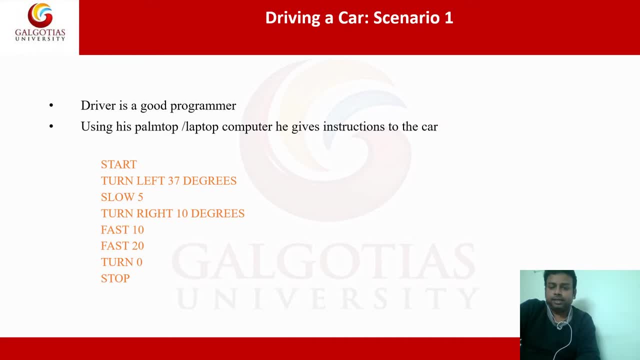 degree. Turn left 37 degree, Then slow five. it will be slow by 5 degree, whatever the unit, kilometer or meter. So the thing is I am getting so here, driver writing a programming and car run all that programs. Okay, So whenever he going to state right, go state in that. 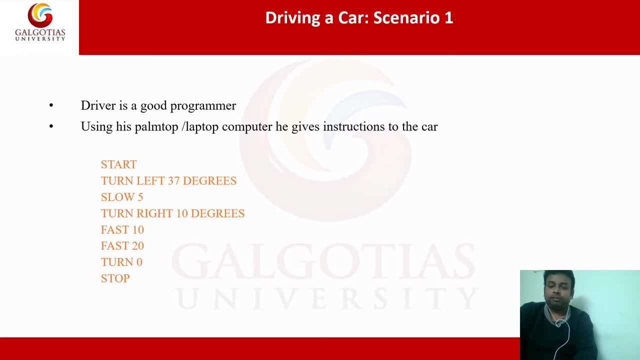 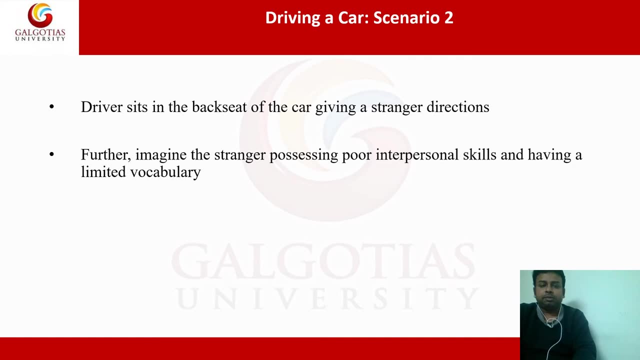 there, then take a left turn. so in that way he is writing some code. basically, another scenario can be possible: driver sit in the back seat of the car and he giving instruction to some other stranger person and on his instruction, stranger person or stranger device run the car. okay, further imagine: 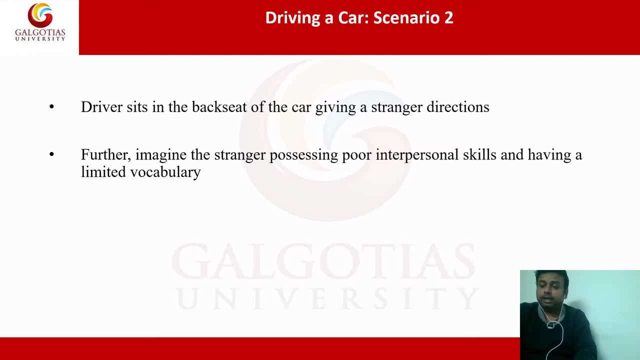 stranger processor may have some poor vocal level, he may. giving some instruction, he may, and the stranger person who actually run the car, he may not understand that instruction. that type of problem can be happened with this scenario. and third scenario is driver himself drive the car by manipulating the steering wheels and paddles. okay, so this is the most natural scenario. 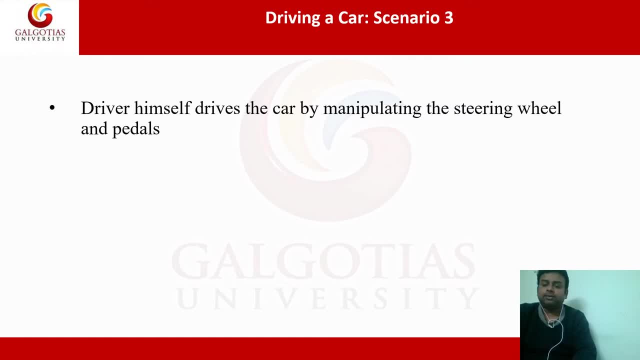 why we discuss this previous two scenario. that scenario is not happened. okay, rarely happened, but this is the most natural scenario whenever we run some four wheeler or two wheeler. okay, but these things also happened. the programming things also happened whenever we run some other car or 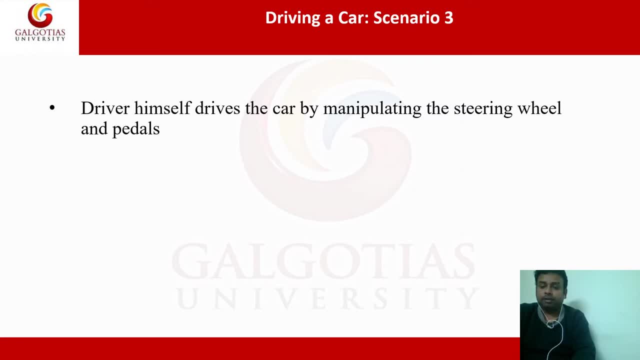 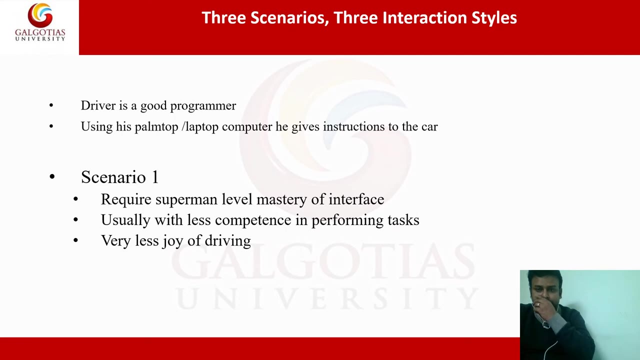 other other type of vehicles, okay, may be happened. okay, so whenever you run one seat, okay, larger seat happen of whenever they are kept at that position. that can be happened, but the problem, the problem with this first scenario, driver have to be a very good programmer and a using laptop or 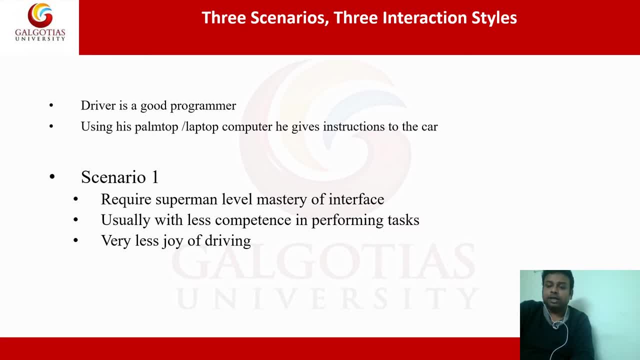 laptop and he give the instruction to the car. okay, this type of scenario driver need to be a very good competency on programming and good develop mastery on the interface. usually with less competence in performance tasks, some problem will be happened and this type of driving driver are not directly drive the car. 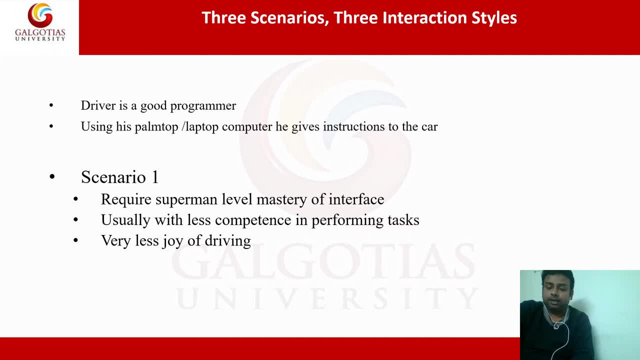 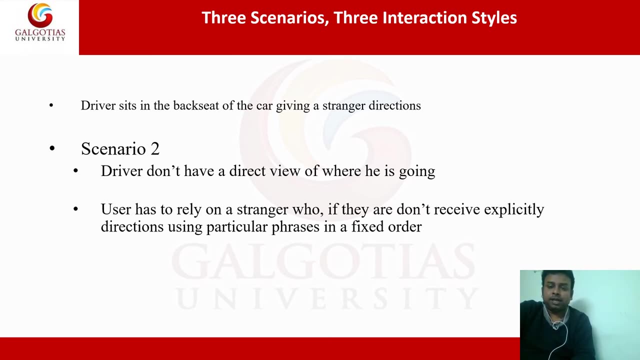 so actually he not enjoy the driving in this type of scenario. okay, he write some program and car is run by that program. in second scenario, drivers sit in the back seat of the car and giving some instruction to a stranger and driver does not direct view where he is going in this scenario. 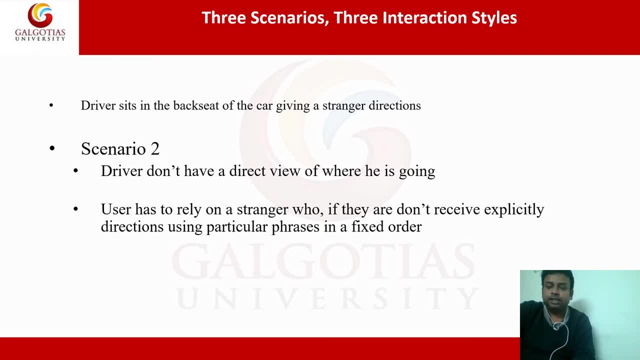 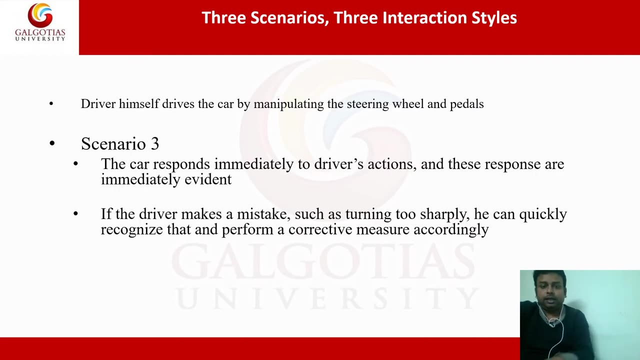 and user has to rely on the stranger who is driving the car. actually, if they are not received explicitly direction using particular phase or order, then some problem may be happened. in the case of our scenario where driver himself run the car by manipulating the wheels and paddles, the car is in this scenario, whatever the car responds. 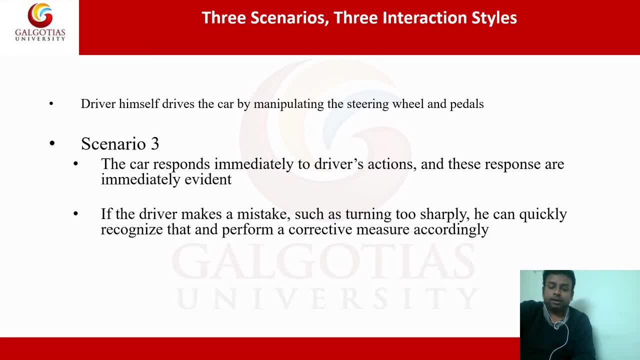 immediately to the driver actions. so whenever, whatever action he taken, that reaction of all from the car is very much immediate and the response are immediately. evident means if you find that turning the car is very, very quick, sharply, then you can understand. okay, I have done a mistake. at the same time, 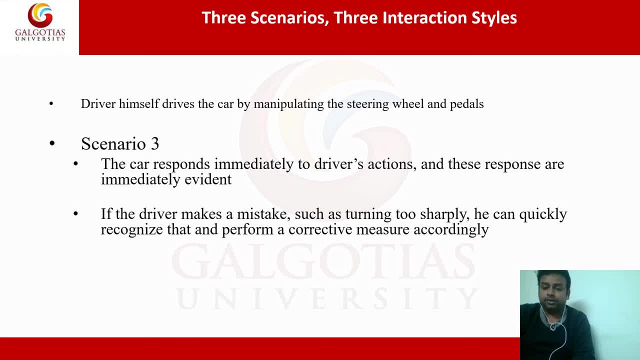 this turning very sharply, okay, so there is a possibility that the car is in this scenario, where the car is in this scenario. so there is a possibility that the car is in this scenario, where the car is in this scenario, where the car is in this scenario, where the car is in this scenario. 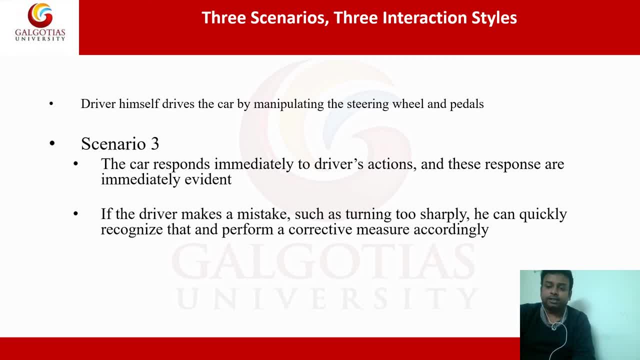 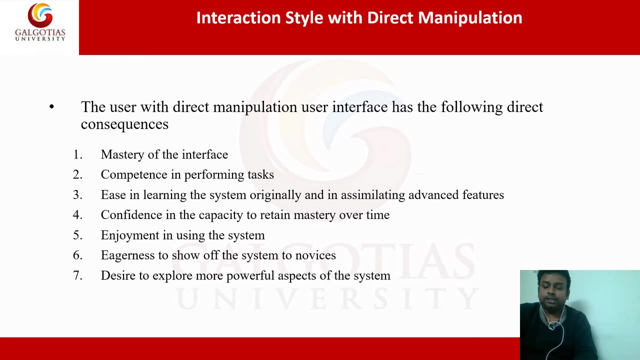 possibility that he can rectify this error, recognize what kind of mistake we have done and the next time we take a corrective action. so this last scenario is the direct manipulation, because we are directly driving the car. so what are the consequence? may be happened with the direct manipulation. so in this type of interaction, 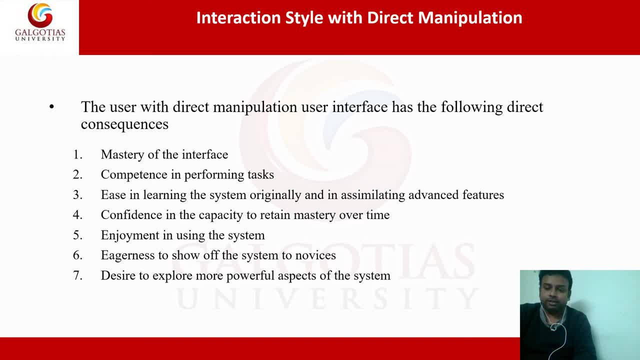 it will happen in mastery of the interface, because we need to run the things, and he will have a confidence in performing tasks. whenever the task is performed, at that time we will get a feedback or he will get the confidence that I am perform the task and it is easy to learning the system originally as in advanced. 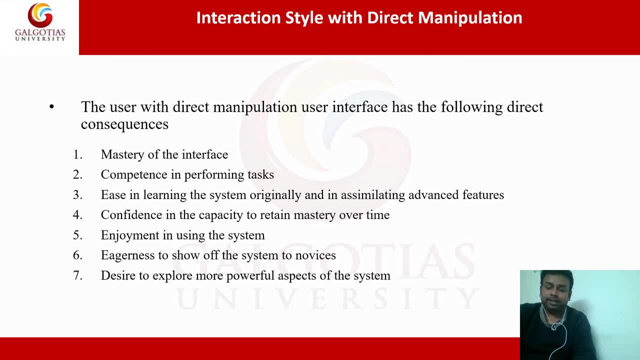 teacher. okay, as it is a directly, you are interacting with the device, so it is something easy to learning and confidence in the capacity to retain mastery over of the time. okay, so by using this, this kind of interaction, several time so you will ultimately get a master level of efficiency on the. 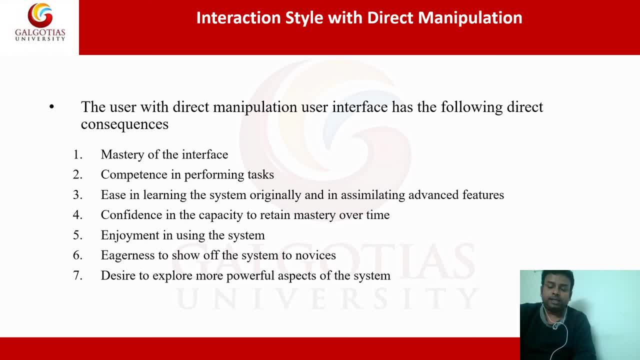 device. so, moreover, in this kind of interaction, you will enjoy the system okay, because the feedback will be in at the same time and you can is to show so. obviously, if you are done by one, then you may have some kind of began this to show the novices and desire to expose more powerful aspects of the systems. 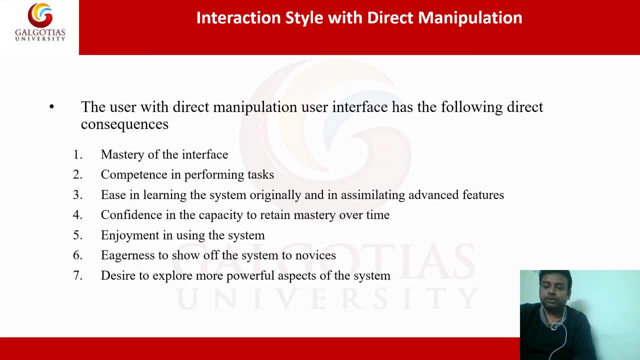 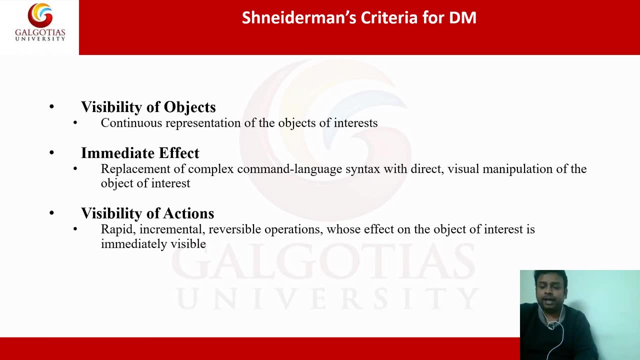 okay, as you directly involved. so there is a chance that we go for more powerful aspect and go for the explore other options also. So there are three different criteria of direct manipulation. That criteria is co-coded by Bates-Zindermann. So first criteria is visibility of the object, continuous representation of object of interact. 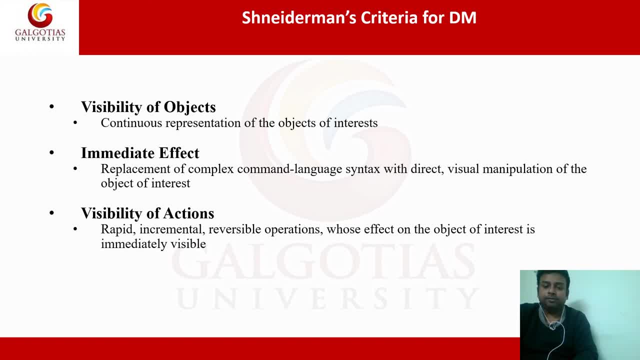 whatever object you need to interact, that object have to be visible. Then immediate effect. replacement of complex format, syntax and direction, visual manipulation of the object of interest. So whenever you performing a task- maybe you perform 5%- had that immediate effect also. 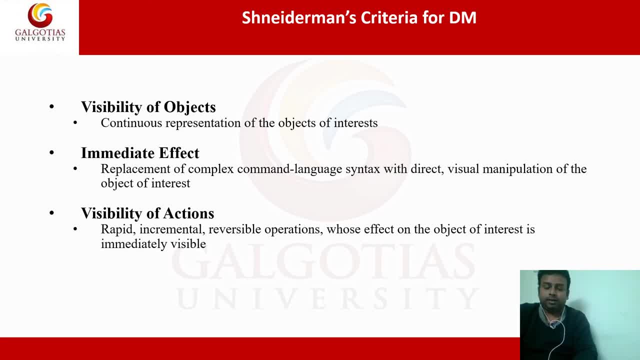 you have seen that after 5% completion what happened? that things also. you show that things also visible to you. Then visibility of the actions: so rapid, incremental, reversible operations whose effect on the object interest visually visible. So after performing the action the effect will be immediately visible. 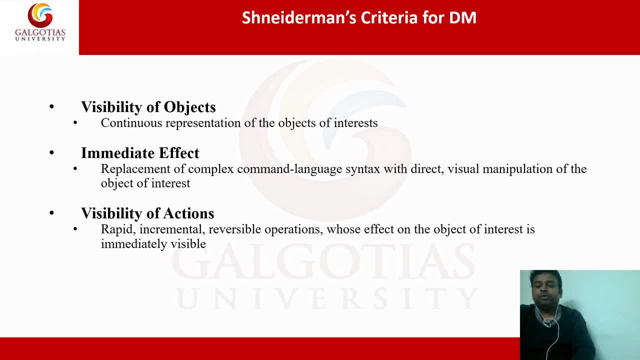 Okay, suppose I am giving one example. suppose you want to delete one object from your desktop. So you want to delete one folder from your desktop. actually, you are deleting to recycle bin. Okay, so for this particular task, how you done. 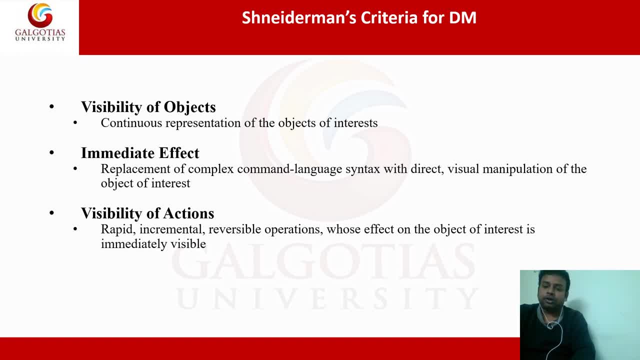 Here in direct manipulation, you go, take your mouse cursor onto the object and drag this thing to the desktop. This is the folder. So basically, whenever you are dragging the particular object, that particular folder, so after dragging some, maybe you have dragged 5% or 10%, so intermediate effect you will. 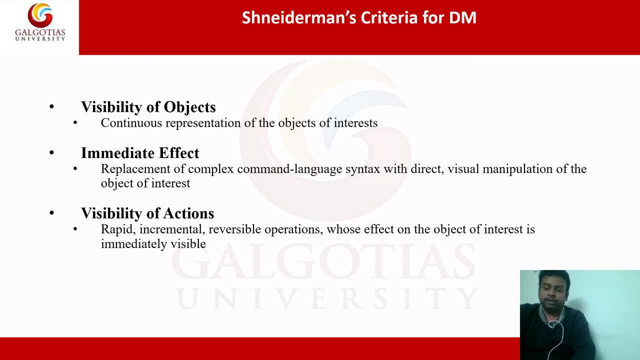 see that particular file will moving from its previous place to the newer place And whenever you drop it into the recycle bin, then you will find out that that particular file are not visible into the recycle bin. Okay, So this is the next step. 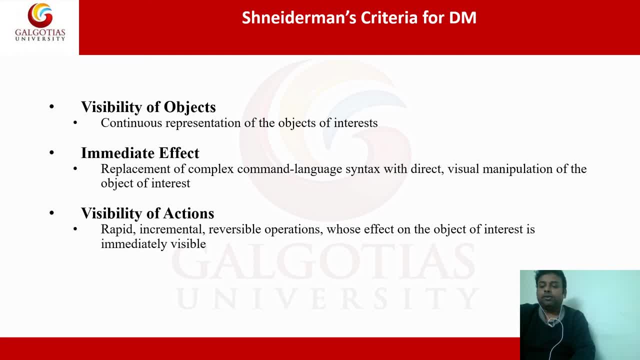 So whenever the task is completed. so visibility of action: okay, we have deleted. Okay, So it is not visible. Okay, So in this, this is an example of direct manipulation. Okay, So further for further reading, you can go with this reference. 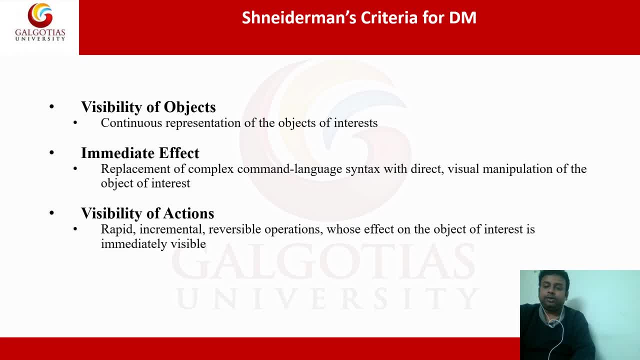